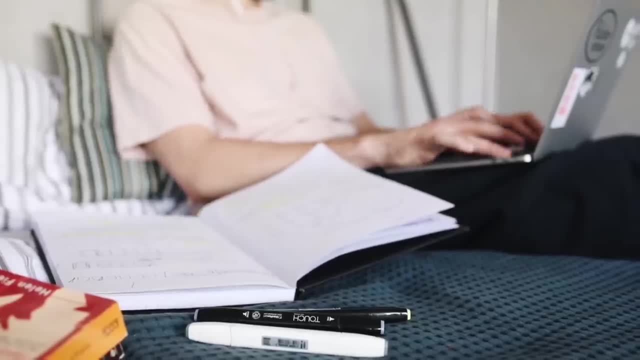 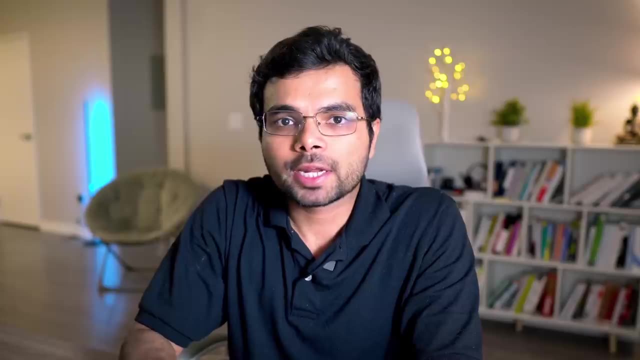 You don't need to go very deep, since most of the learning will happen while solving coding challenges, But make sure you are familiar with how to calculate the time and space complexity of an algorithm using Big O Notation. Learning Big O Notation will help you improve your algorithms and better understand why. 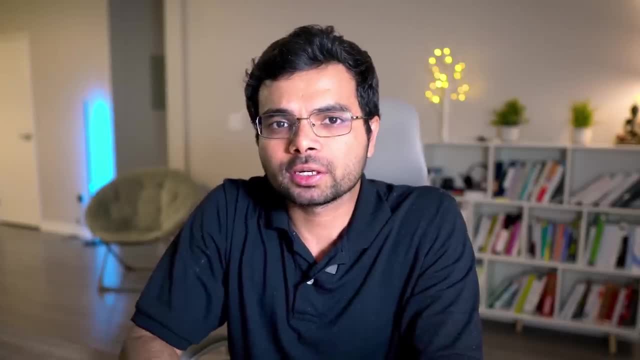 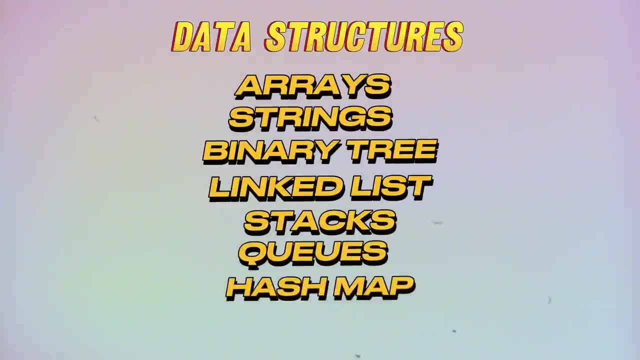 your algorithm may be running slowly. Once you have a grasp of Big O Notation, familiarize yourself with fundamental data structures like arrays, strings, binary trees, linked lists, stacks, queues and HashMap, And learn basic algorithms such as sorting, searching and recursion. 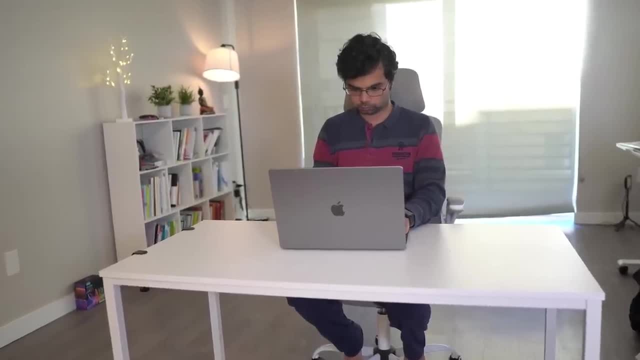 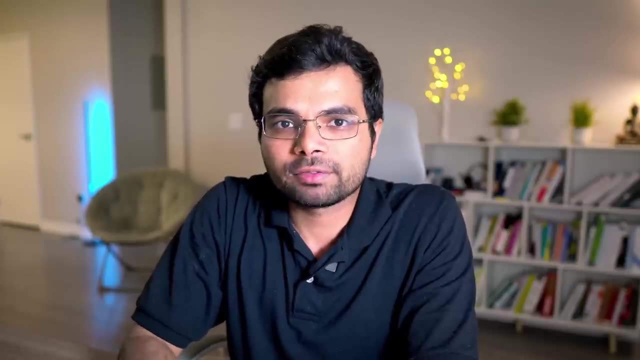 You don't need to know advanced concepts, but it's important to know how to implement basic concepts in your preferred programming language. To learn these topics, you can find many resources online. One YouTube channel that I found particularly helpful for learning data structures is William. 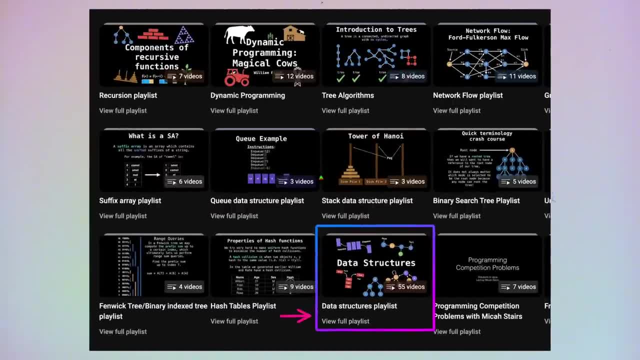 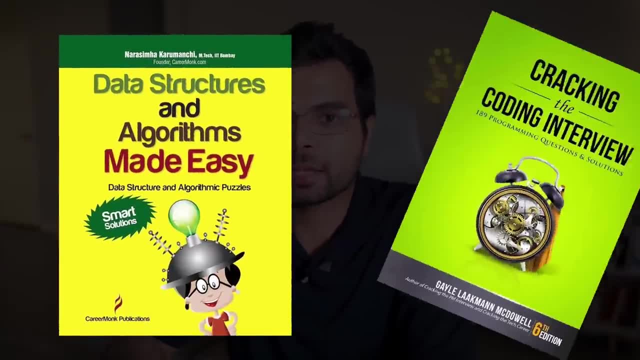 Fissett. They have a data structure playlist where important data structures are explained visually. If you like reading books, then I recommend reading Data Structures and Algorithms Made Easy by Narasimha Karumachi and Cracking- the Coding Interview by Gail Laquman McDowell. 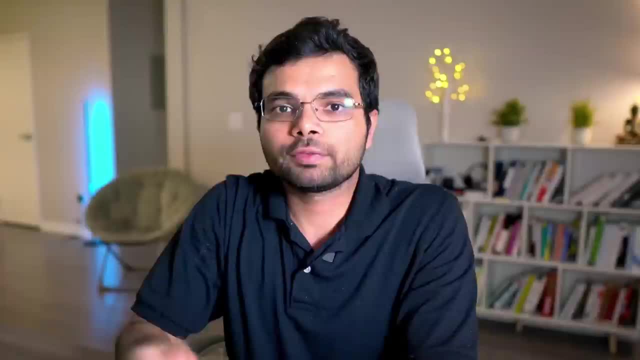 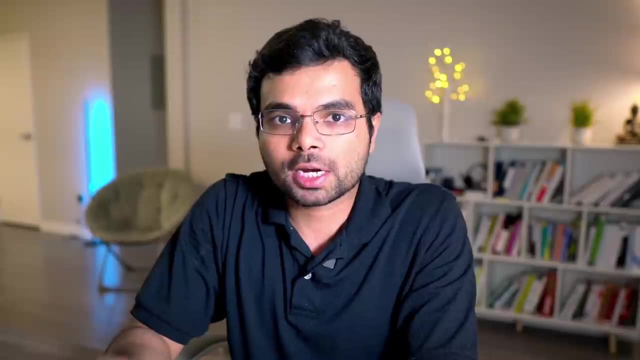 There are thousands of problems on leetcode. Which ones to solve? If you are a beginner, start by studying the following. Start by solving problems by topic. This approach will help you gain a deeper understanding of each topic and learn which data structure or algorithm to use for a specific problem. 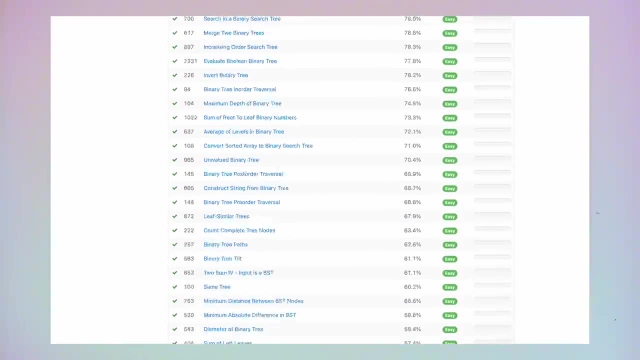 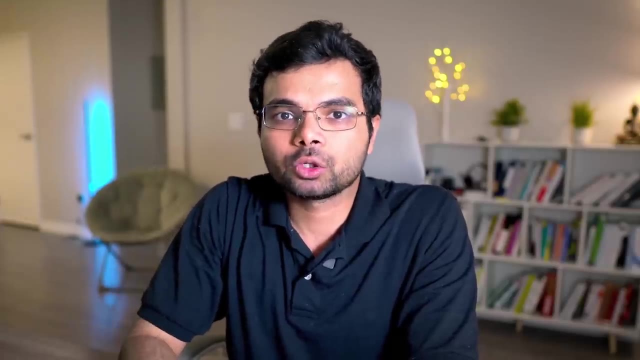 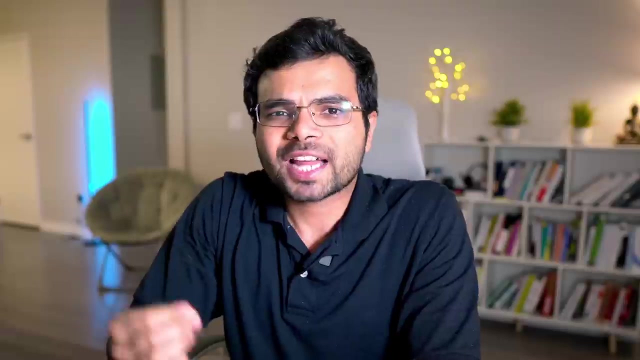 For each topic. start with easy problems. Once you can comfortably solve easy ones, slowly start challenging yourself with problems which are slightly outside your comfort zone. You must constantly challenge yourself to get better. Don't worry about hard problems in the beginning. In most interviews you will encounter medium-level problems, so focus most of your time on those. 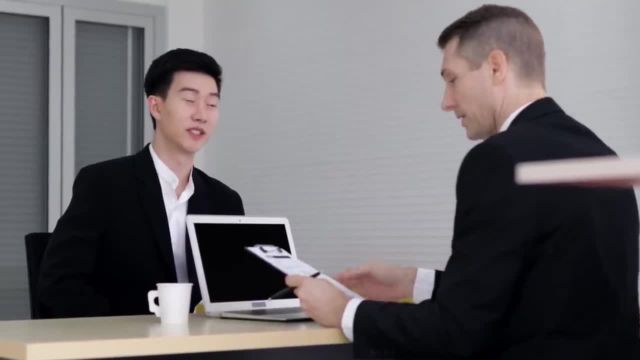 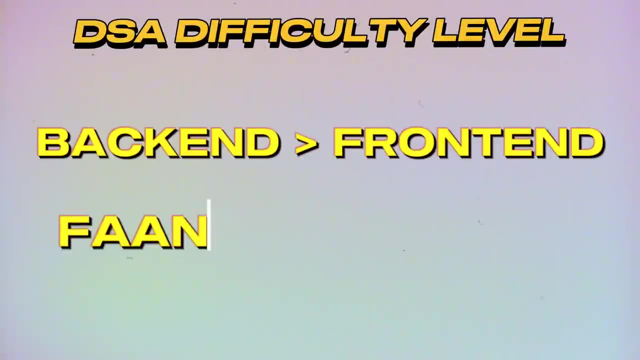 The types of problems asked in interviews differ from company to company and it depends on the role you are interviewing for. In general, back-end roles tend to ask harder questions compared to front-end roles, And FAANG companies ask no difficult questions compared to start-ups. 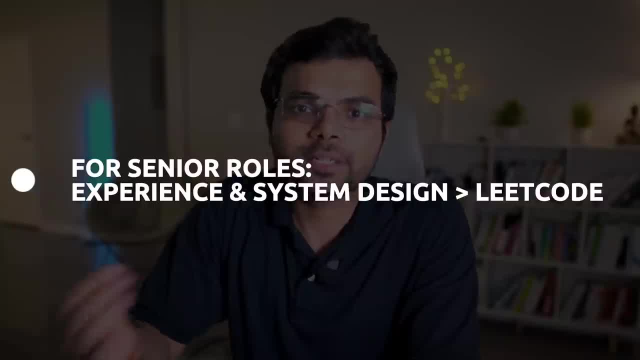 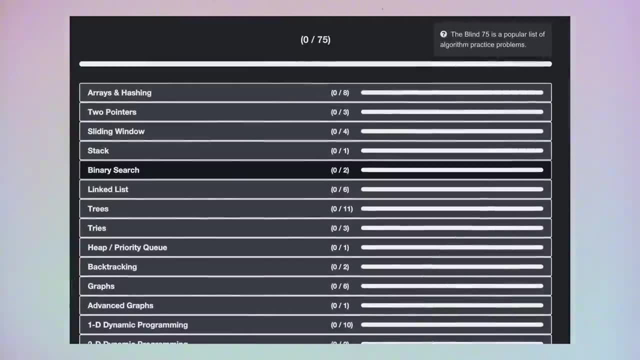 For senior roles, experience and system design matter more than leetcode questions. If you already have some experience with leetcode or similar platforms, you can choose curated lists of problems like neetcode 75 or top 100 liked or top interview 150 questions on. 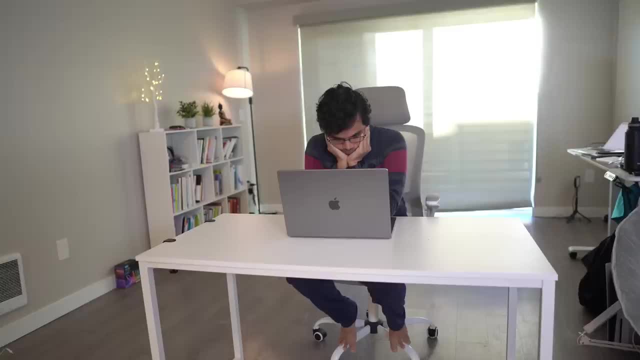 leetcode. Don't spend too much time on highly disliked questions. They will drain your energy and demotivate you. Sometimes you may come across a problem that you don't want to solve If you don't know how to solve it. you may have a problem that you don't know how to. 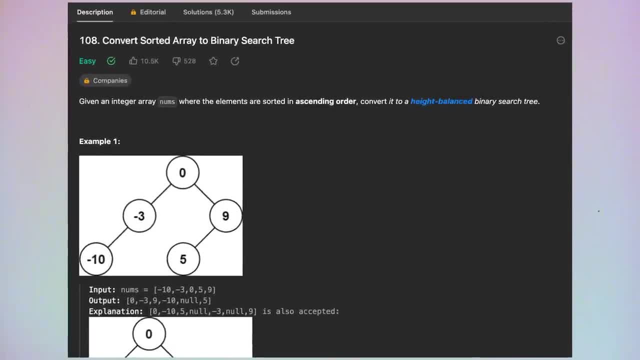 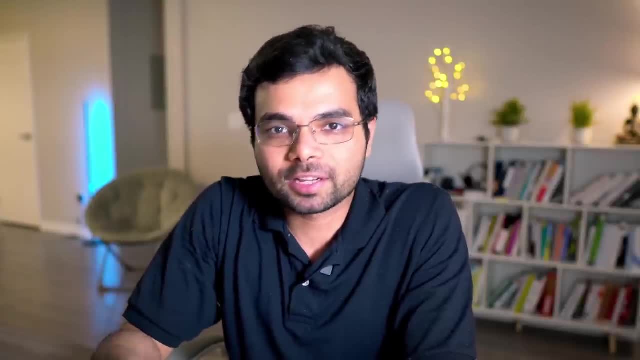 solve. You may have a problem that is tagged as easy but still proves to be difficult to solve. Don't get discouraged. This is all part of the learning process, and sometimes leetcode doesn't do a good job of classifying the difficulty level of the problem. 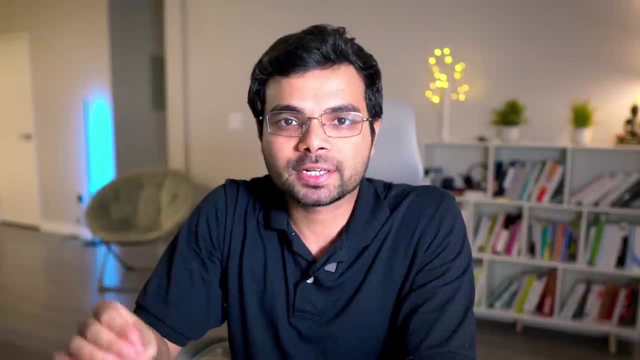 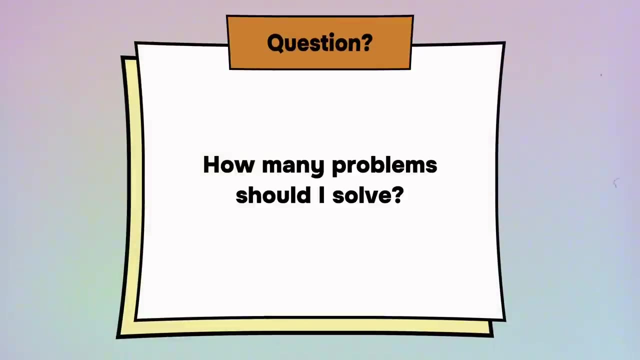 Avoid jumping between problems too quickly. Give each problem sufficient time and effort. After every problem you solve, ask yourself: what is one thing knowing which made everything else easier? How many problems should I solve? This is subjective and depends on the level at which you are at. 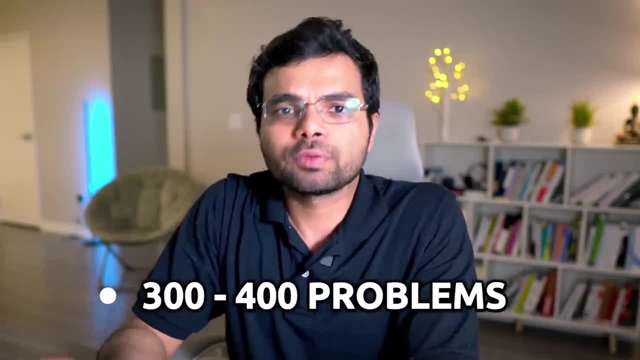 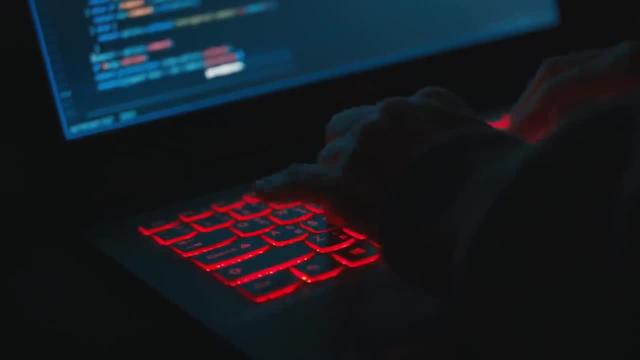 If you are new, you would need to solve more problems- In general, 300 to 400 problems. A mistake I made in the beginning was rushing to increase my problem count without spending enough time on each problem. Instead of focusing on the quantity of problems you solve, focus on what you learn from each. 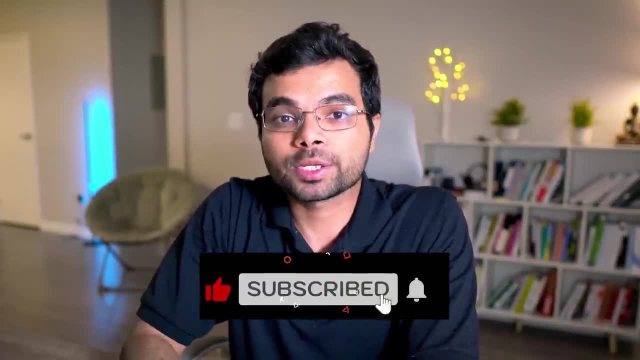 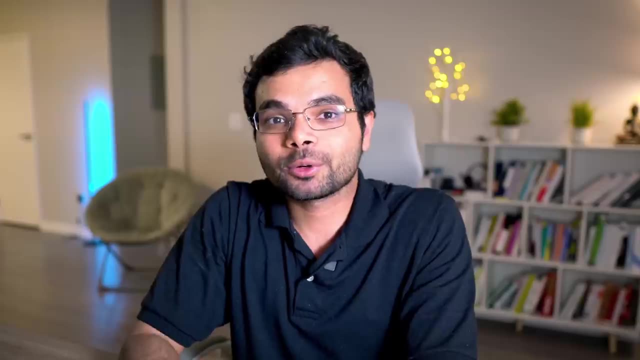 problem. It is much better to thoroughly understand and solve 20 problems than to solve 100 problems without much understanding. Also, try to make it fun. There is a fun in learning to solve coding challenges. It's not just about getting a job. 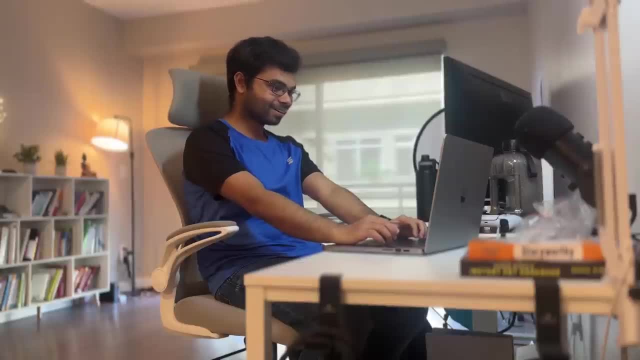 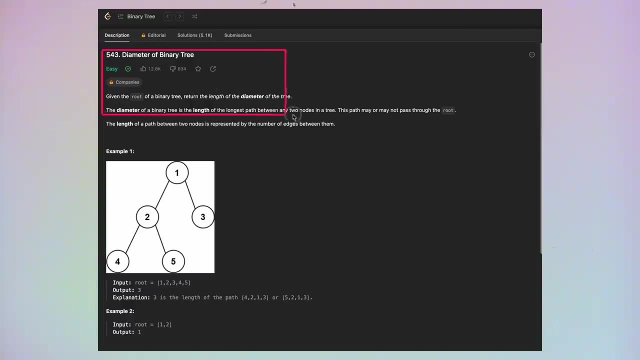 I was able to solve such a high number of problems because I enjoyed challenging myself and felt excited whenever my solution was accepted. How do I approach a new problem? Take some time to understand the problem statement and the expected input and output patterns. Write it down on paper, if it helps. 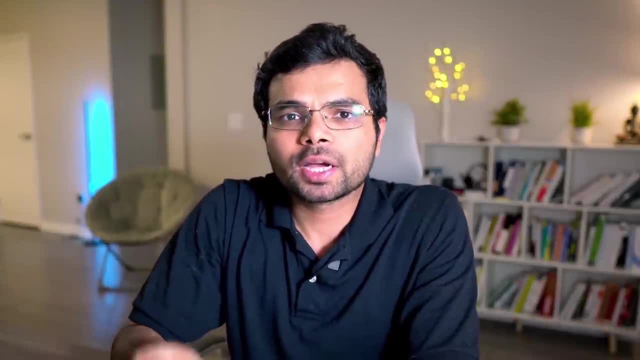 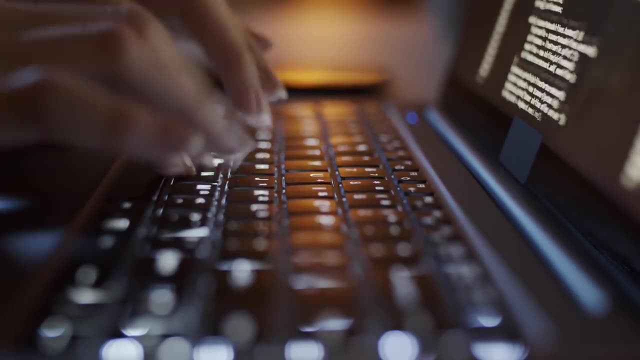 Start with a brute-force solution and then work on optimizing it. Think about how you can improve the algorithm or reduce the time and space complexity. Plan your approach before coding. Coding is easy once you know what you are going to write. So before writing a single line of code, make sure you understand what exactly you are going. 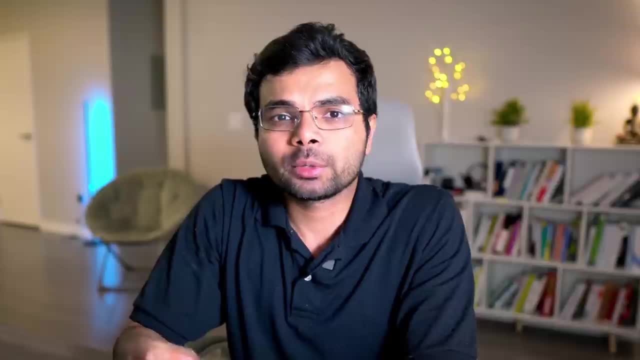 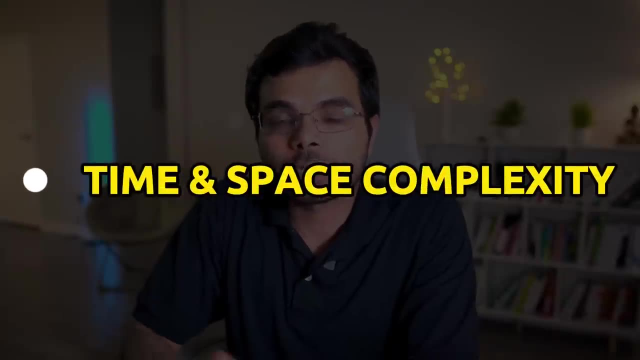 to write. That's one reason why programming language doesn't matter much, Because it doesn't take too long to implement a solution. Once you have a good idea on what to write, develop the habit of analyzing the time and space complexity of every problem you submit. 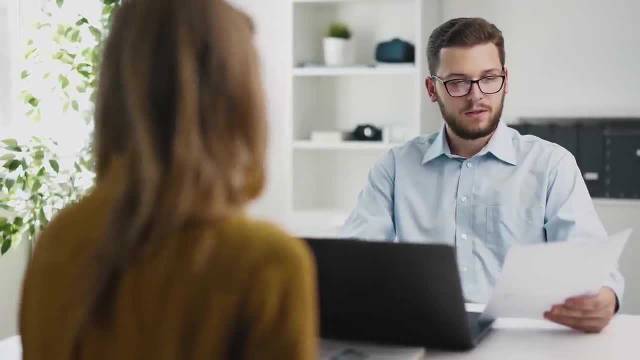 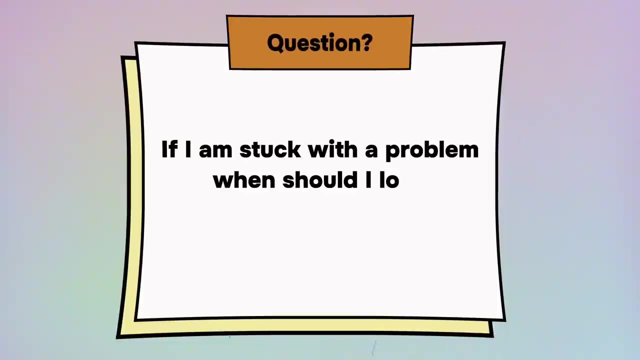 Interviewers focus a lot on finding optimal solutions and may ask about the complexity of your code. It is a good practice to test your code with small inputs, including edge cases. If I am stuck with a problem, when should I look at the solution? 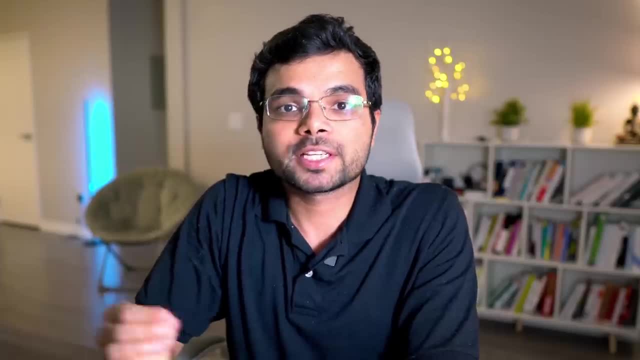 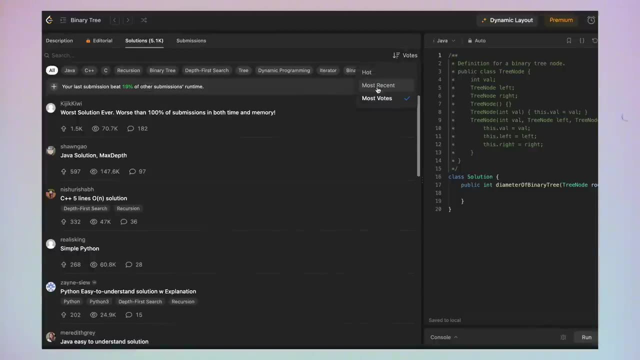 Give at least 30 to 60 minutes of focused effort to a problem. If you are still stuck, look at hints and solutions. Don't spend too long on one problem. Read the official solution And try to understand the top-rated solutions. 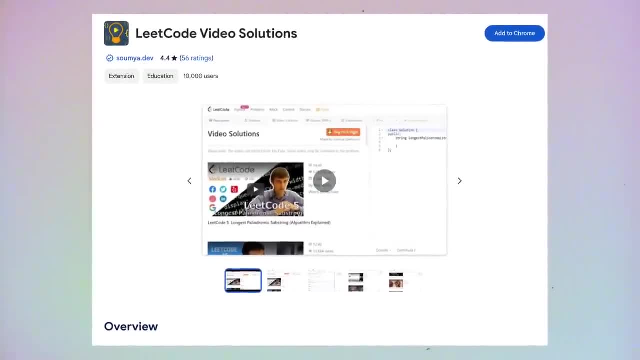 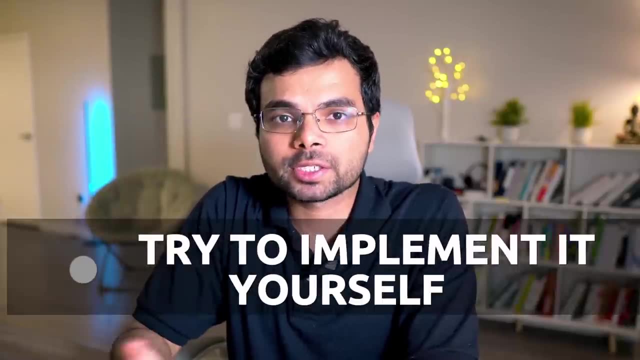 You can check out this extension called Leetcode Video Solutions, which allows you to watch solution videos directly on the problem page. Don't just move on. after being the solution, try to implement it yourself. Also, since you were able to solve this problem on your first attempt, it's a good idea to 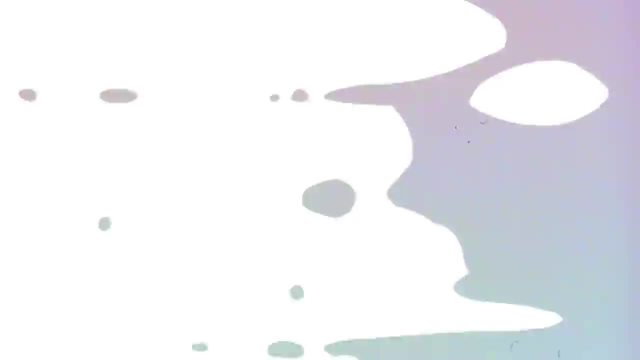 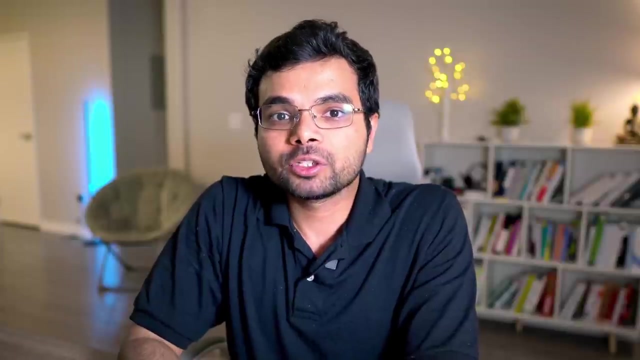 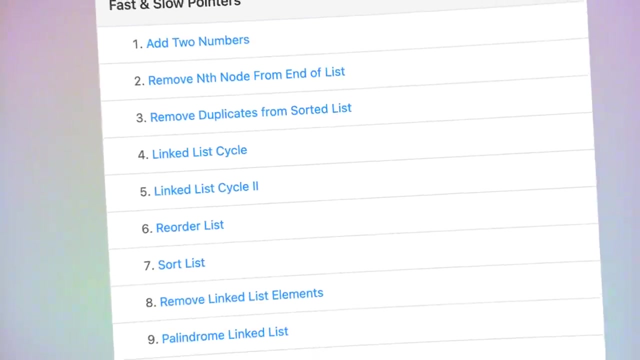 market for revision and revisit this problem after a few weeks. Question: How do I solve more problems in less time? The answer is to learn patterns. Instead of focusing on individual questions, Concentrate on the problem. Learn identifying patterns On Leetcode. you will come across multiple problems that follow a similar pattern. 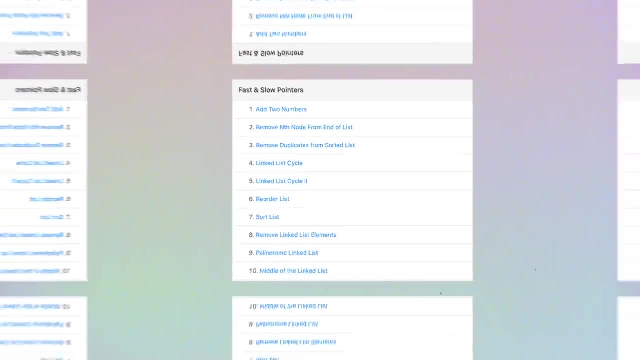 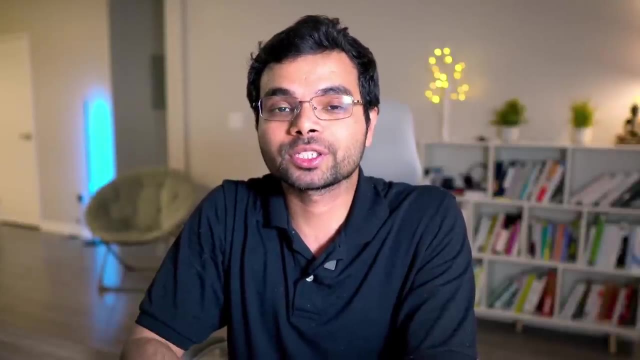 Once you know how to solve one of them, you can apply the same approach to solve others. For example, after learning this sub-string pattern, I was able to successfully solve more than 20 sub-string questions using the same approach. I have created a GitHub repository to list common Leetcode patterns from different articles. 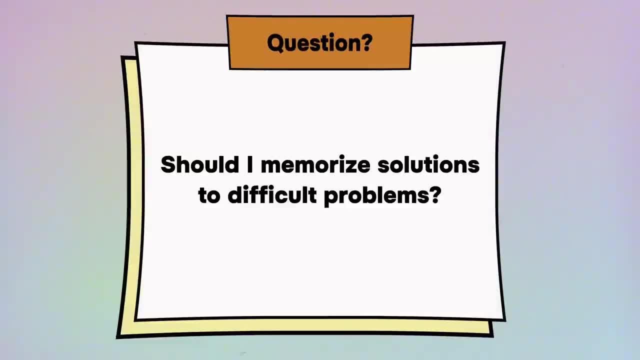 You can find the link in the description. Question: Should I memorize solutions to difficult problems? When I was a beginner, I used to memorize the solution to the difficult problems. I used to memorize the solution to the difficult problems. When I was a beginner, I used to memorize the solution to the difficult problems. 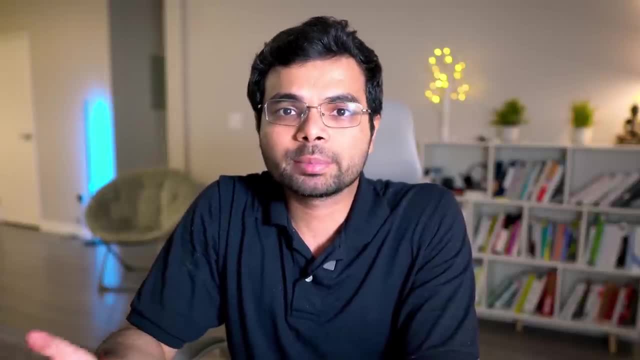 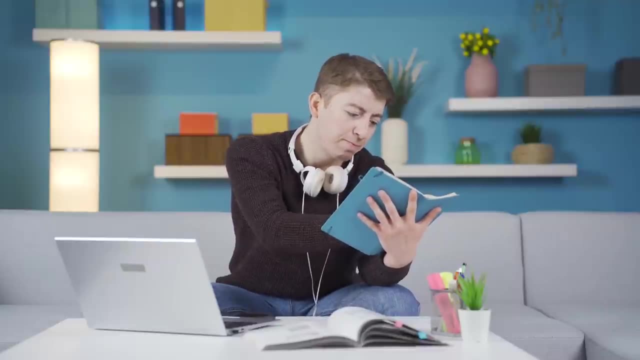 I used to memorize the solution to the difficult problems And move on. I later realized that it was a big mistake. Memorizing solutions does not improve your problem-solving skills And it is not helpful during interviews, Because the interviewer might ask a variant of the problem or a follow-up question. 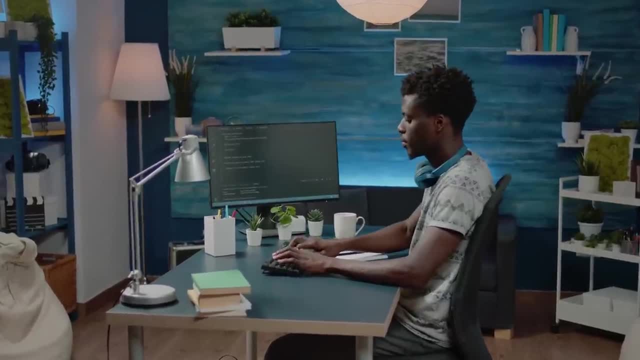 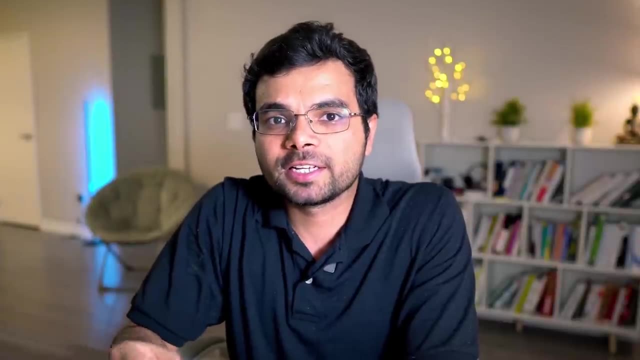 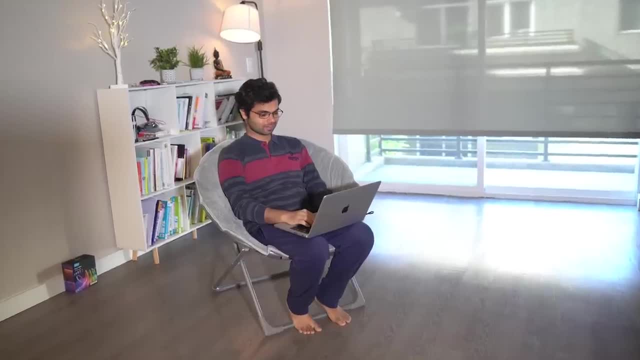 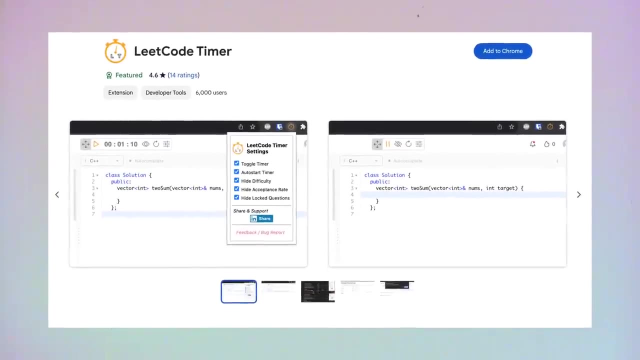 Solving a problem during an interview is very different from solving it at home, sitting at your sofa. That's why you need to practice in a timed environment. There is a Leetcode extension called Leetcode Timer that you can use to time yourself while practicing. 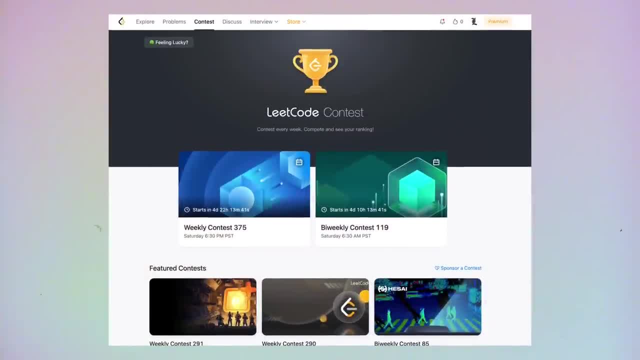 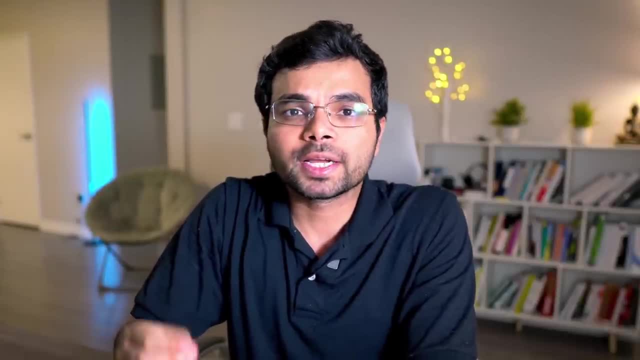 I highly recommend participating in Leetcode contests, as they provide the best way to practice in a timed environment. Don't worry if you struggle to solve even one problem in the beginning. The whole point is to gain some experience solving problems within a time limit. 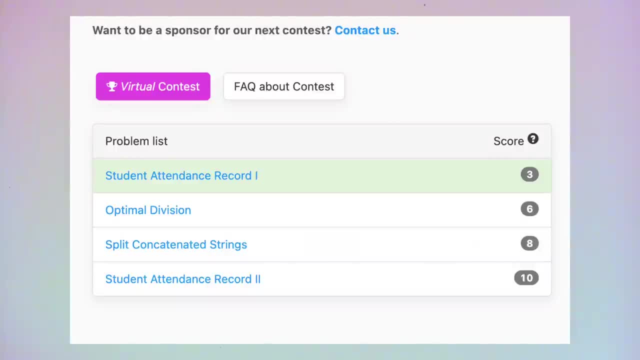